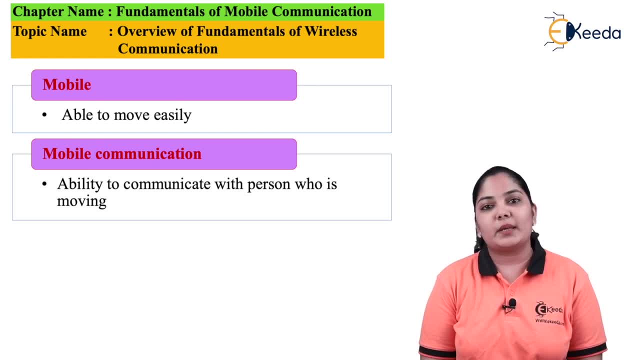 that I am able to communicate with the person who is able to move freely. When we talk about the term mobile, it means I am able to move freely about communication. what is that we really want to communicate? we want to communicate voice, and not only voice. in today's world, we want to communicate data as well. when we talk about 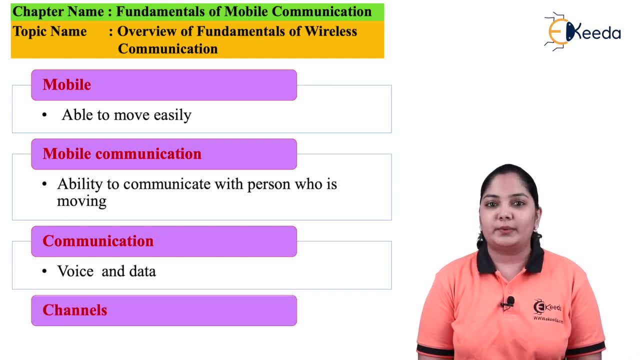 wireless communication systems. what is the channel that we are really talking about? since it is wireless, the channel is free space, meaning, if it is a free space, there is a lot of noise that is going to add to this channel. what are the various noises that could be added? it could be either a. 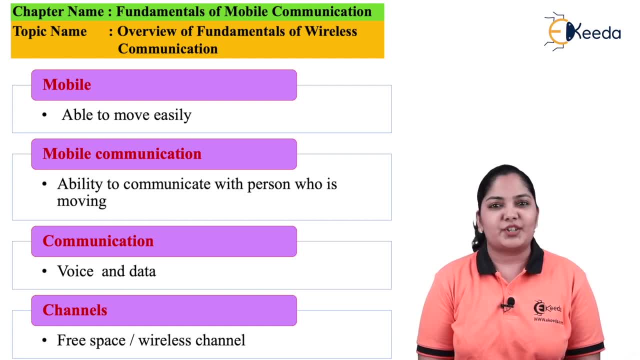 natural noise or a man-made noise? what are natural noises? maybe the radiations from the sun, maybe the cosmic noise from the stars or lightning in a thunderstorm. various man-made noises, like industrial noises, sparkling or lightning of automobiles, could also add as noise into this channel. 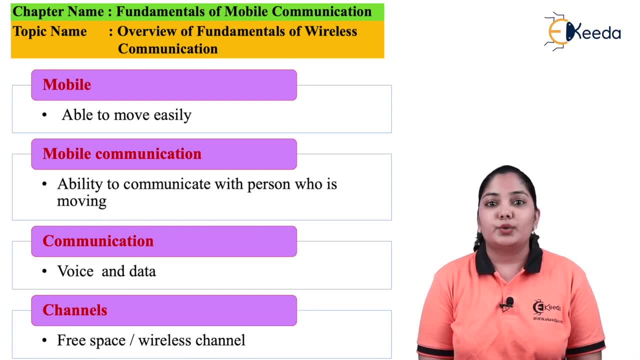 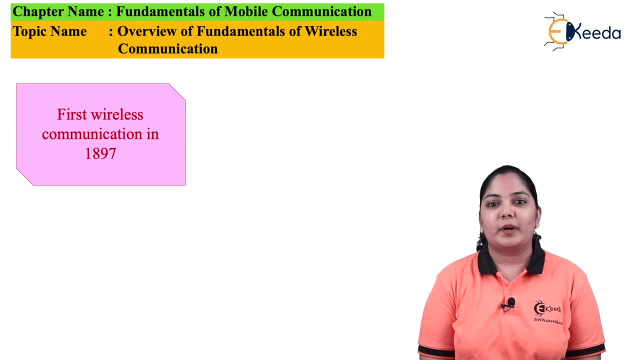 and hence it is very important to design all the transmitters and receivers in a way that we are able to suppress the noise and transmit our voice and data with correctness. the first wireless communication system was shown by marconi. what he tried to show was that the ships that were 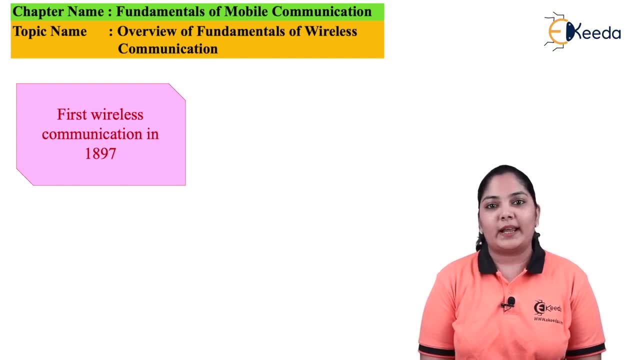 sailing in the english channel were able to make contact using frequencies and hence the improvement in the English channel was able to make contact using frequencies and hence the improvement in English channel was able to make contact using frequencies and hence the improvement of various rf and radio circuits started. improvement of digital circuits started, as we all know, large-scale. 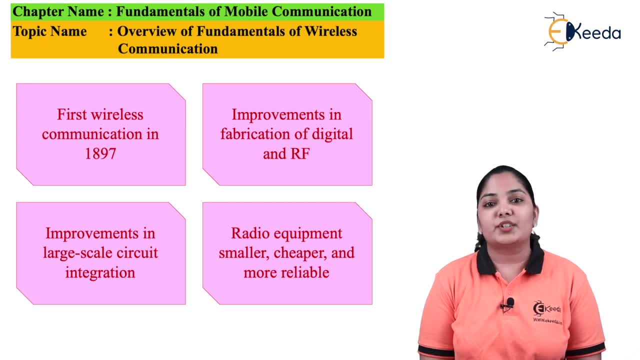 integration circuits started when the industrialization started. today we talk about vls i, which means very large scale integration. we're able to mount huge amount of components on a very smaller chip. this made the mobile equipments very slow and those which are being smaller, and because digital communication was used for transmitting and receiving data.